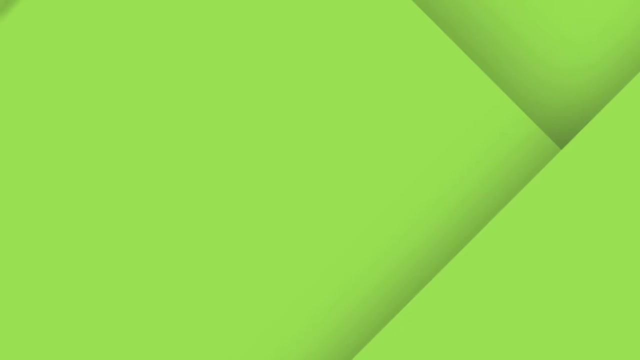 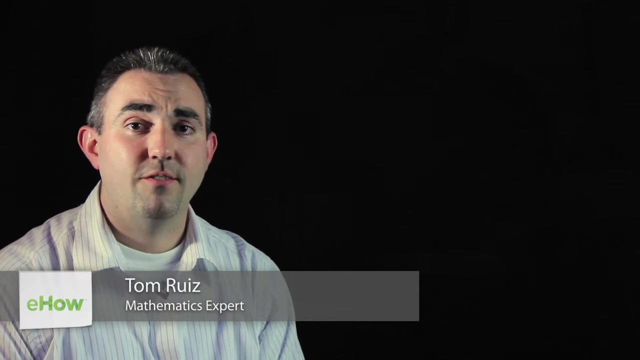 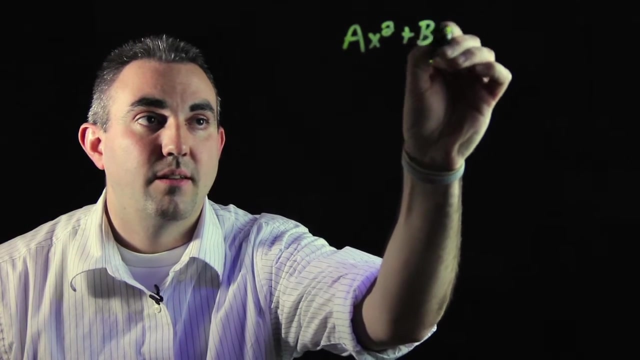 Hi, I'm Tom Ruiz and I'm a math supervisor. Today we're going to discuss how to write a quadratic equation given three points. The standard form of a quadratic equation is ax squared plus bx plus c equals y. Now you're going to be given three points, and your first- 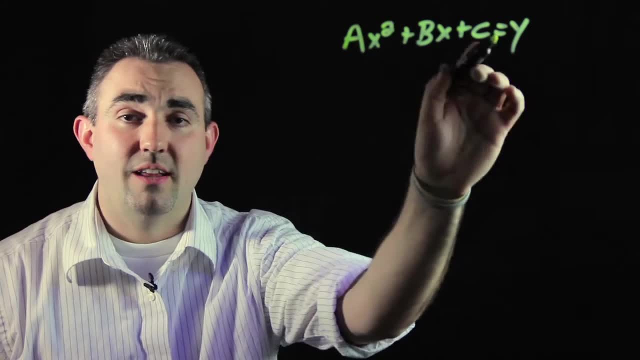 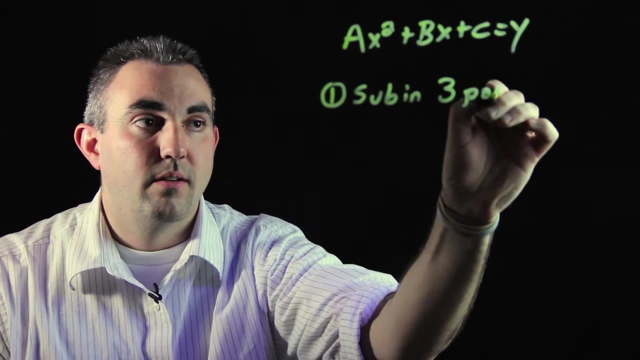 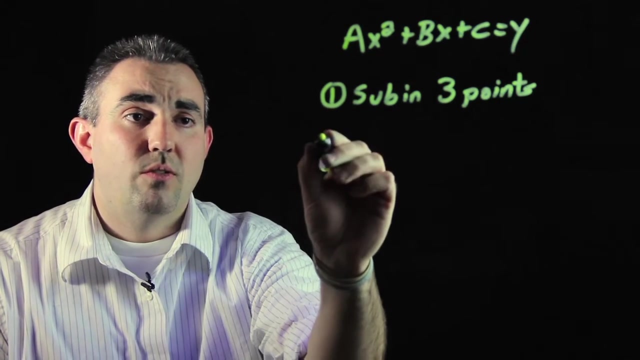 job is to substitute each one of those points individually into this equation. So step one is to sub in three points. When you do this, you're going to get three separate equations. What you need to do with those three separate equations is use the elimination method to 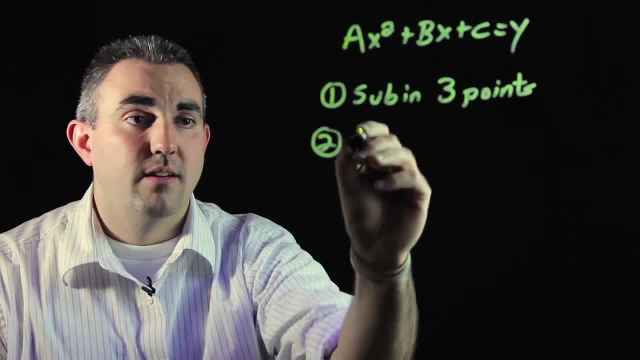 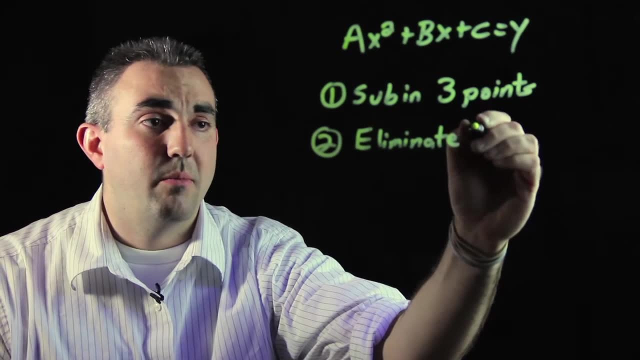 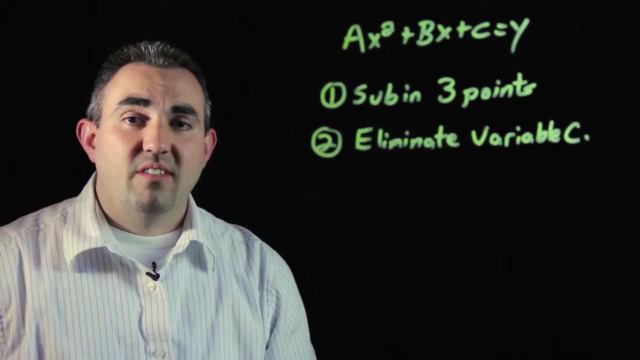 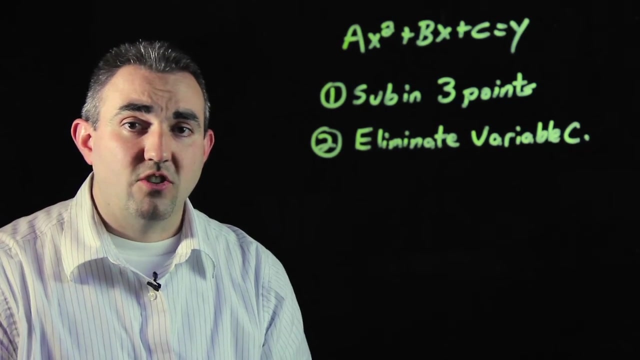 get rid of one of the variables, either a, b or c. Let's say we're going to eliminate variable c. When you eliminate variable c, you'll have two brand new equations that only have an a and a- b. You need to take those two equations and use the elimination again to get rid of. 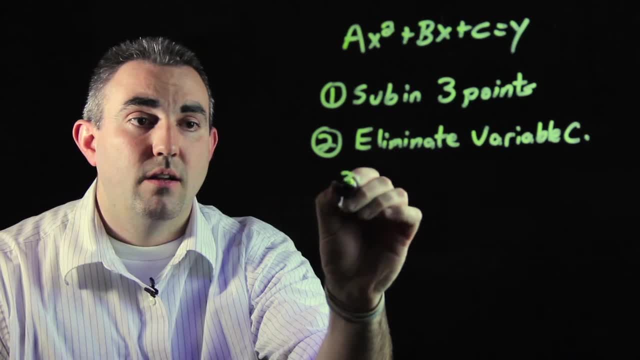 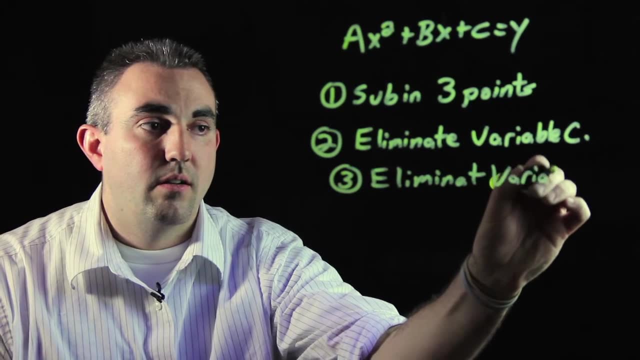 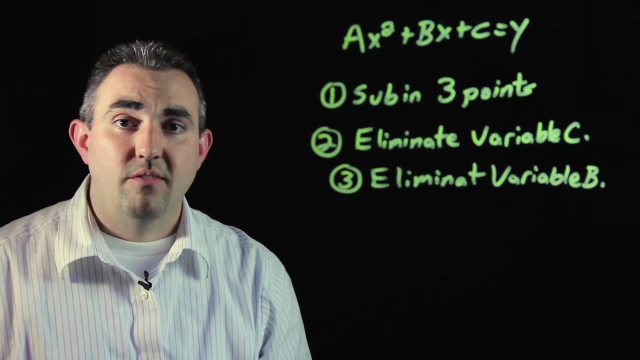 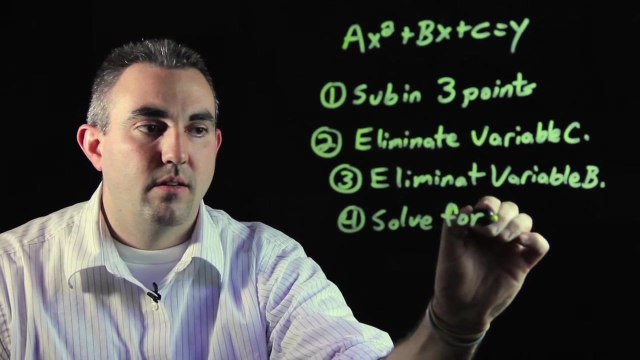 either a or b. Let's eliminate variable b. Step three: eliminate variable b. Now you have an equation with just one variable, Variable a, which you can solve for. Solve for a. Now you're going to take a, your answer. 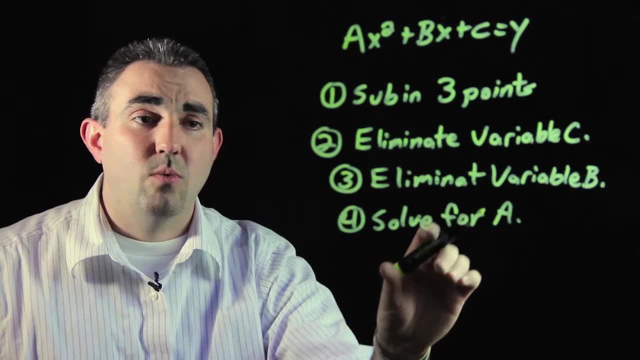 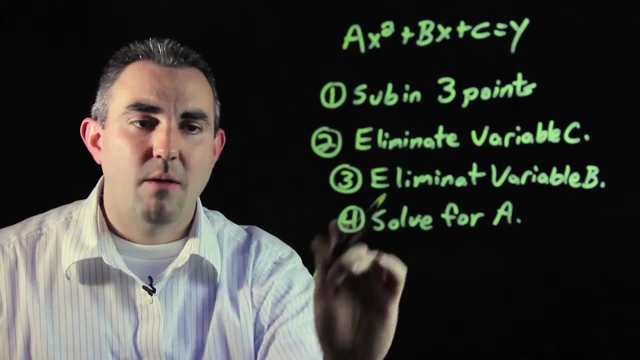 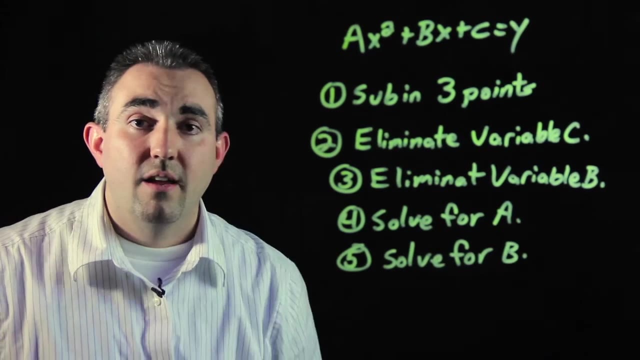 that you have for a and you're going to sub it back into one of the equations that you got after we eliminated variable c, One of those two equations that we have. stick a back into that and solve for b. you have A and B. What you're going to do with A and B is take it and sub it back into. 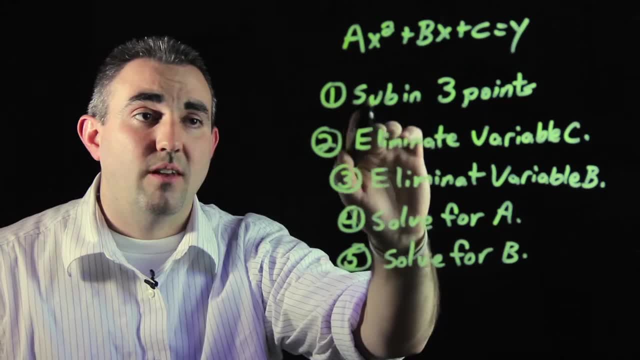 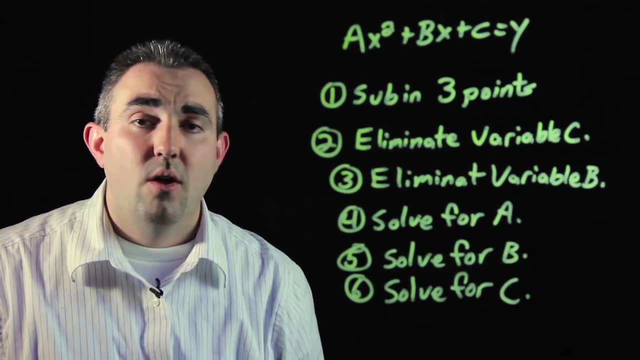 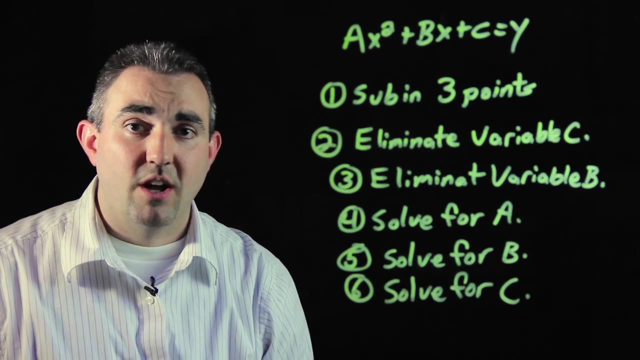 one of the original equations that you got after you subbed in your three points. So step six: solve for C. Once you have A, B and C, you can plug them back into your standard form equation for a quadratic. I'm Tom Ruiz, You do the math. Subtitles by the Amaraorg community.